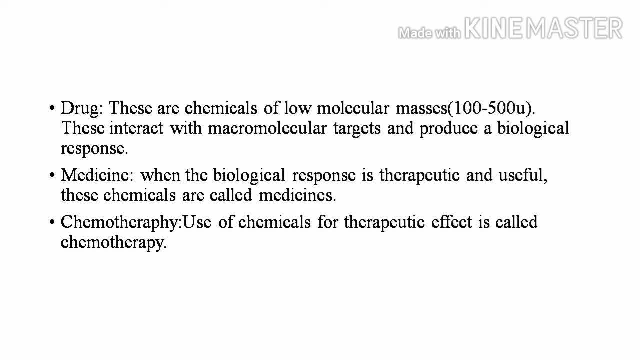 as a macromolecular target. whenever the chemical interact with this micromolecular target, automatically there is a cure. is there then that chemical which is used to reduce the effect caused by bacteria or virus or virus or any other microorganism is called as drug. so let us try to understand once again. 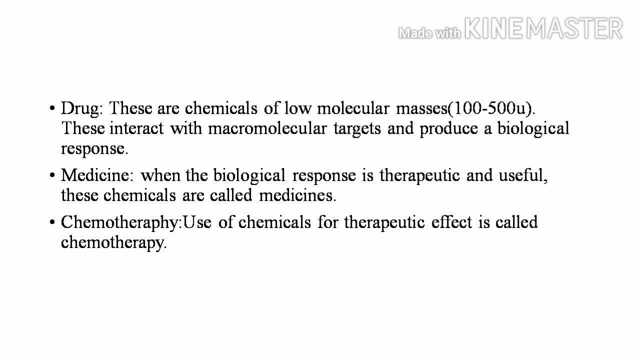 drug is the chemicals of low molecular masses. these interact with macromolecular target to produce a biological response. now you may have a doubt: what is biological response? biological response means see, whenever you got temperature, doctor advise you to take the paracetamol. so what happens? when you take the paracetamol, the body temperatures start decreasing. so that is. 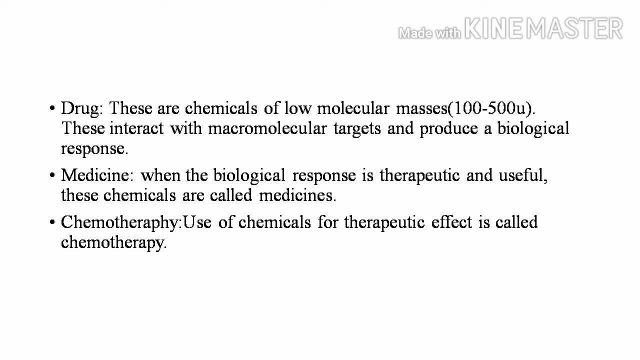 called as a biological response. now let us try to understand about another important term: medicine. when biological response is therapeutic, therapeutic. what is meant by therapeutic, therapeutic means which is used to cure a disease? so medicines are where the drugs which produce biological response is therapeutic and useful. these chemicals are called medicine. I repeat: when the biological 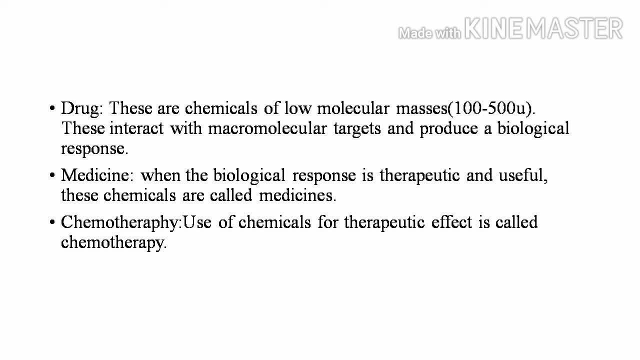 response is therapeutic and useful. these chemicals are called medicines. That means these medicines are useful in order to diagnose, in order to cure and in order to prevent the disease. So medicines are useful for three different ways. One diagnosis: that means 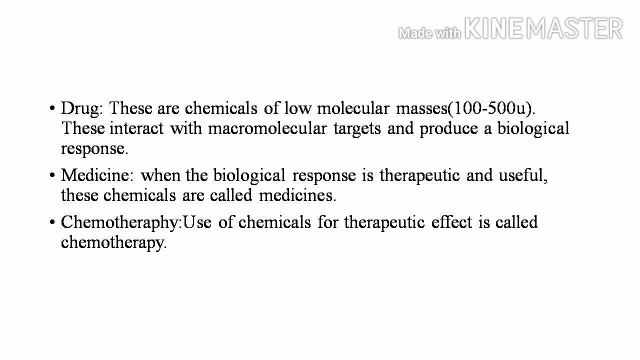 identification. Two: cure: that means in order to cure the disease. Three, to prevent: that means see when you have taken the vaccines. those vaccines are useful, so that they cannot. the disease may not again occur again and again If you have the polio vaccine DTT. 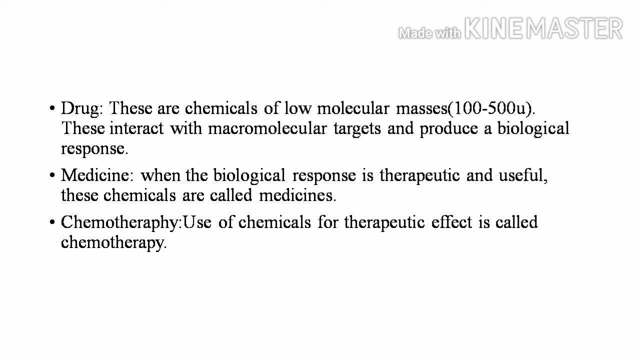 and all others. right Now let us try to understand about chemotherapy. Use of chemical for therapeutic effect is called as chemotherapy. Chemotherapy means when medicines are used to identify, to cure and to prevent the disease. that process is called as chemotherapy. So 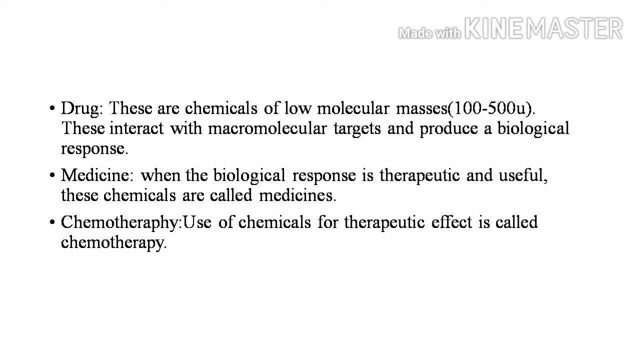 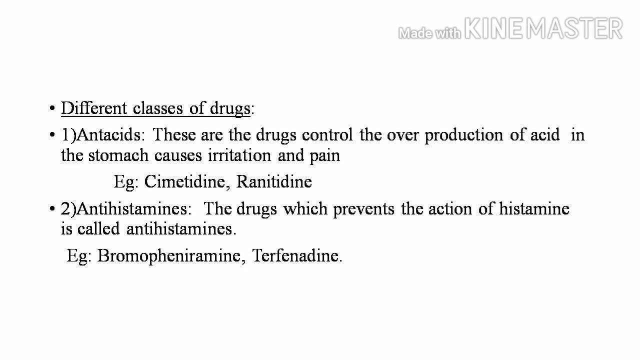 chemotherapy involves three different stages: One identification, Two treatment, Three prevention. So chemotherapy. So chemotherapy involves three different processes: One is identification, Second one is cure, Third one is prevention. Now let us try to understand different types of drugs. 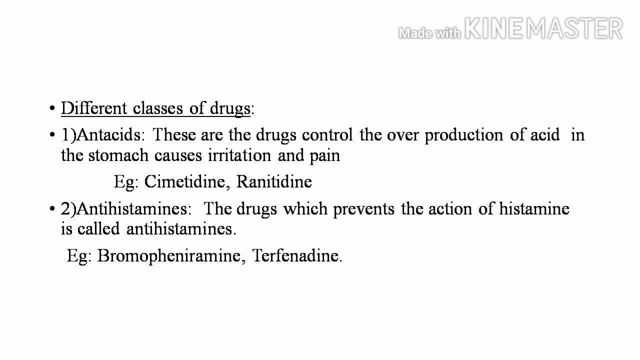 and their classification. First let us try to understand about antacid. These are the drugs control. the overproduction of acid in stomach causes irritation and pain. See, when you have eat so much of sore food, then after some time our stomach got irritated. 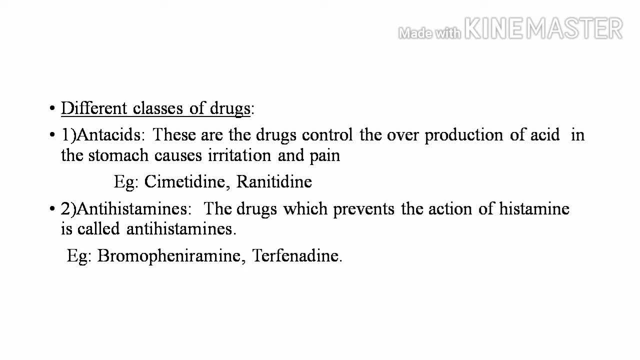 and we are going to have so much of pain In order to reduce the pain. when you have taken a soda, or when you have taken a you know, or whatever the ads which are coming on our TV whenever you have taken it, automatically our stomach pain. 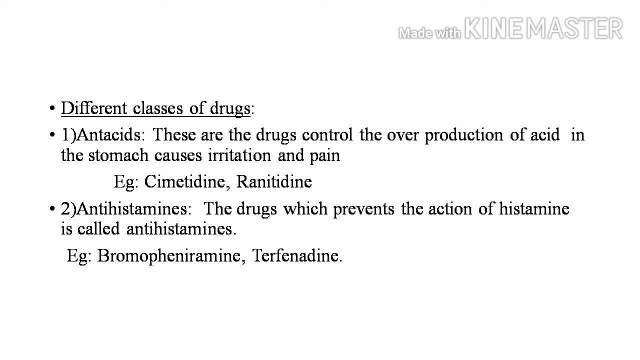 got to decrease. Do you know why Those antacids are, you know? or those find acid available in the market? They are nothing but the mild bases. whenever the mild base is taken in the form of liquid, that interact with the excess acid produced in. 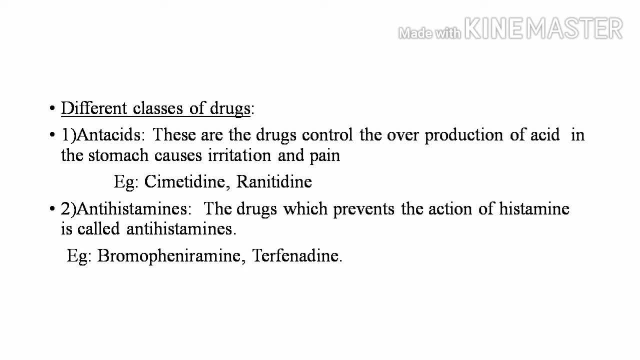 the stomach and control the excess acid produced in the stomach. So antacids are the drugs which control excess acid produced in the stomach. I repeat: antacids are the drugs control over production of acid in the stomach which causes irritation and pain. Example of these antacids is simitidine. 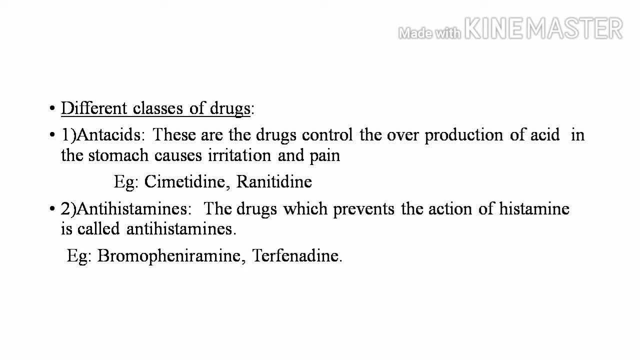 and rantidine. Now let us try to understand about antihistamine. These drugs which prevent the action of histamine, is called as a antihistamine. When the histamine interact with the walls of the stomachIt causes so much of pain, This leads to ulcersSo antihistamines are. 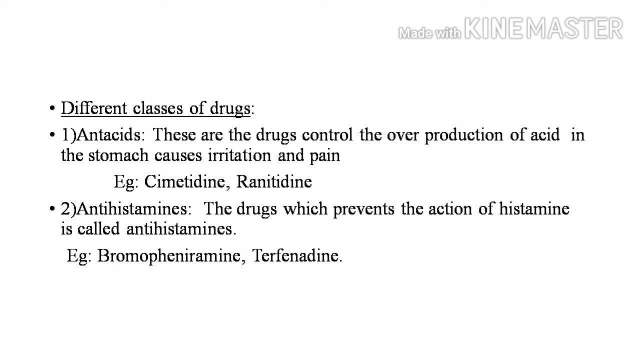 the drugs which prevent the action of histamineOr antihistamines are the drugs which prevent interaction of histamine with the body. Why do we believe tamilk not to have tistamine in women As a body? Severe women are not perfect. 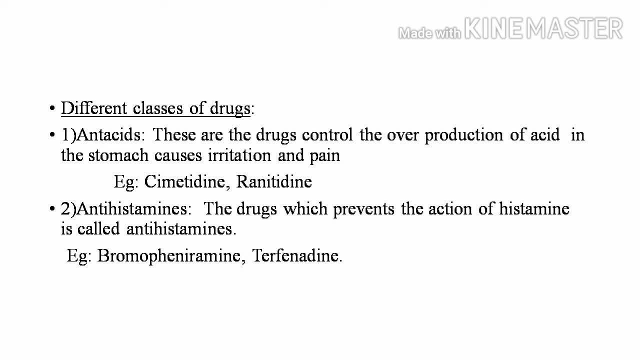 unfair to your pregnancy? It is not if it is not before the individual jerk you get. some walls of stomach are called as a antihistamine. example of antihistamine are bromopherine and teriferine. now let us try to understand about tranquilizers. 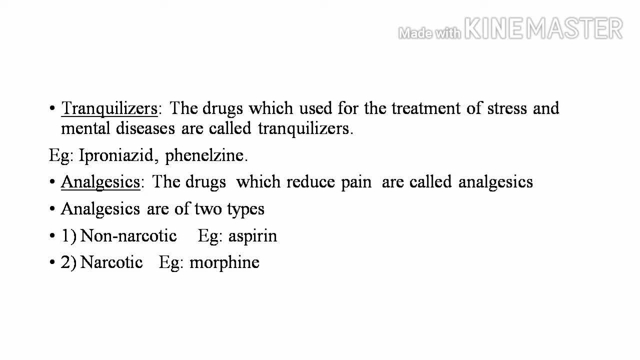 the drugs which used for treatment of stress and mental disease are called as tranquilizers see so recently you have seen the death of Sushant Singh Rajput, who who had committed suicide because of stress, and there are so many mental diseases are there which can be cured very easily by using tranquilizers. so 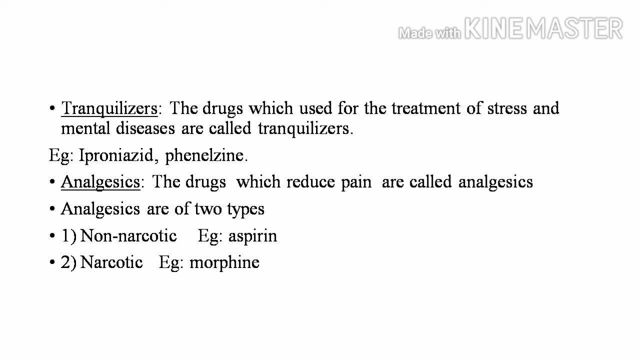 tranquilizers are the drugs which used for treatment of stress and mental disease are called as tranquilizers, so tranquilizers. measure a is to relax the excited mind. so in order to come calm down those stress, in order to relieve the stress, I personally suggest to do yoga and meditation. next, 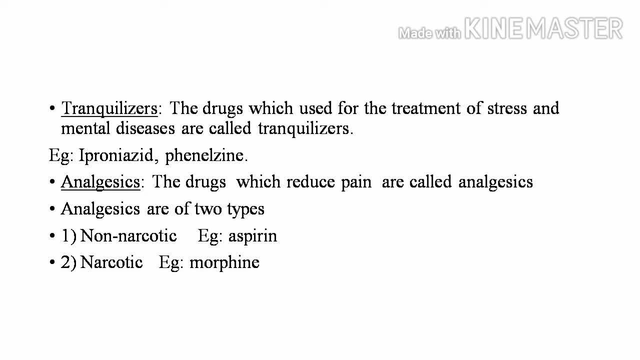 let us try to understand about analgesics. analgesics are the drugs which reduce pain. I repeat, the drugs which reduce pain are called analgesics. analgesics are broadly classified into two categories: they are non-narcotic drugs and narcotic drugs. first, let us try to understand about non-narcotic. 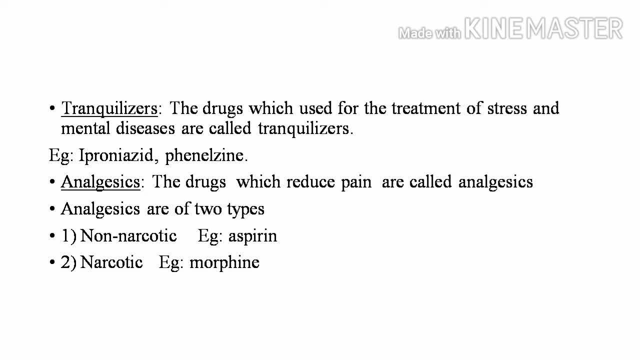 drugs. see, when a person is there who is having so much of anxiety to smoke, if you stop that person also, he won't listen to us. he used to have the habit of smoking. that means he won't listen to us. he used to have the habit of smoking. that means 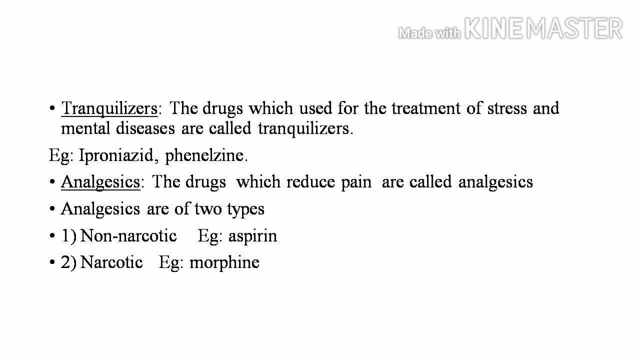 means here. he has addicted to it. so there are some persons are there who are taking the cocaine. those are giving relaxation. those are giving relaxation towards your pain. but if you have taken that drug for a long time it affects the central nervous system. so narcotic drugs are the 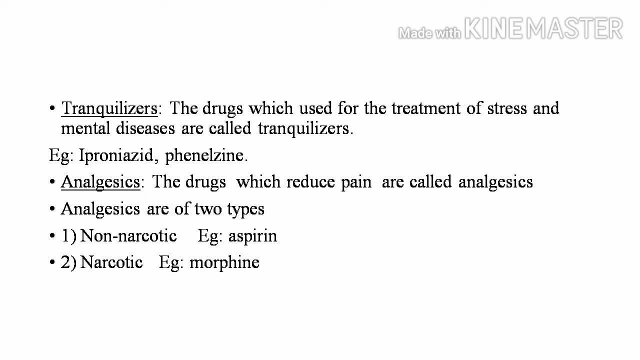 drugs which relieve pain, but after taking them for long time, which causes harmful effect. those are called as a narcotic drugs. example of narcotic drug is a morphine codine, cocaine and all others. next let us try to understand about non-narcotic drugs, the drugs which are used to reduce pain. 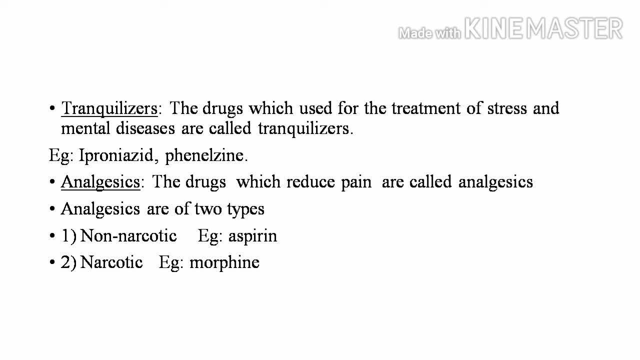 even the drugs is taken for a long time. also, it may not cause much harmful effects to central nervous system- are called non-narcotic drugs. that's why, without having doctor advice, i request all of you don't take any medicine, because taking medicine for longer time will always affect our human body. 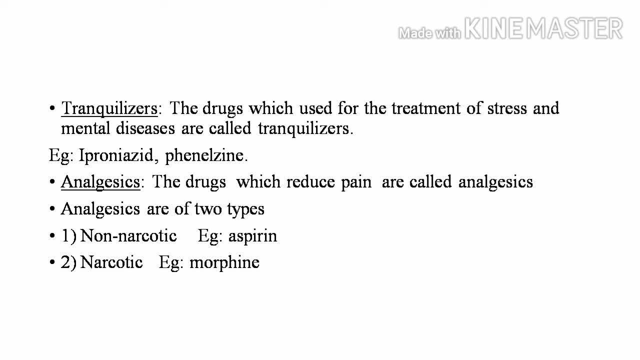 so analgesics are broadly classified into two categories. they are narcotic drugs and non-narcotic drugs. narcotic drugs are the drugs which relieve pain, but if those drugs are taken for a long time those may affect central nervous system, whereas non-narcotic drugs are the drugs which relieve pain, even though if they are taken for 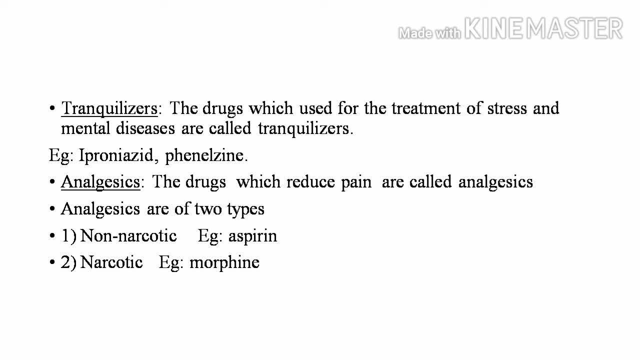 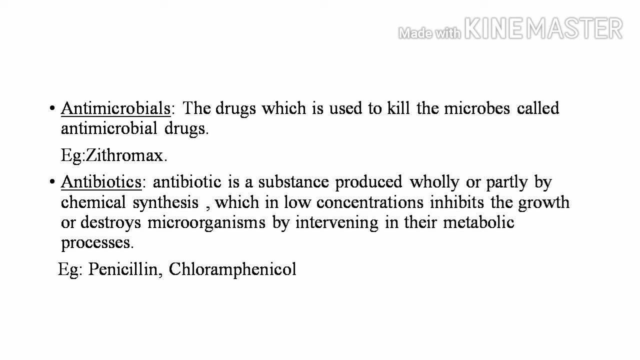 long time. also, they may not cause any harmful effect to the human body, are called as a non-narcotic drugs. next, let us try to understand about antimicrobial, the drugs which is used to kill the microbes, called antimicrobial drugs. because of certain microbes, our body gets affected, so in order to treat that disease, 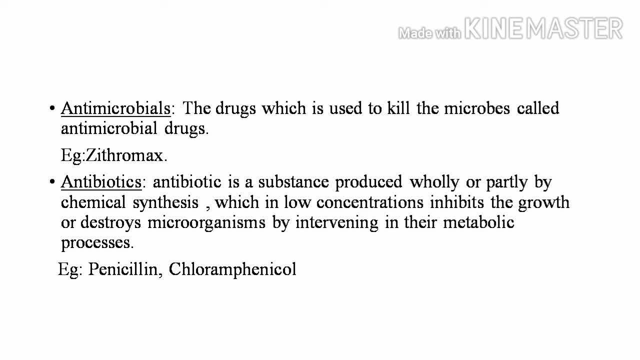 we are going to take the antimicrobial drugs. so antimicrobials are the drug which is used to kill the microbes are called anti microbial drugs. so antimicrobial drugs are the drugs which is used to kill the microbes are called antimicrobial drugs. example, as antimicrobial drugs are: zitromax. 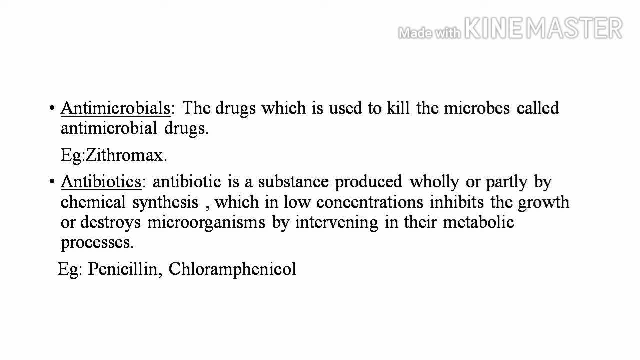 next, let us try to understand about anti biotics. I think all of you have learnt about do great scientist Alexander Eagle Flaming, who had introduced the penicillin. So what is antibiotic? Antibiotic is a substance produced wholly or partially by chemical synthesis which, in lower concentration, inhibit the growth or 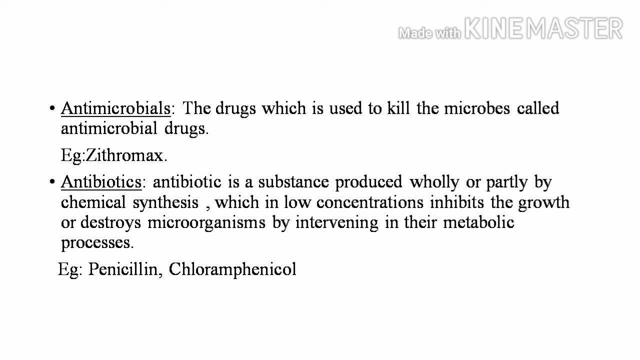 destroy microorganism by preventing in their metabolic process. Simply, I will say this: antibiotics are the drugs which are produced from microorganisms and used to kill the microorganisms. I repeat: antibiotics are the drugs which are produced from a microorganism and used to kill. 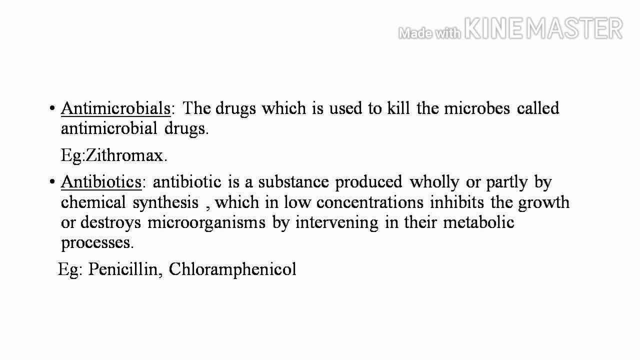 the microorganism. So those are called as antibiotics. I repeat: antibiotics is a substance produced wholly or partially by chemical synthesis which, in low concentration, inhibit the growth or destroys microorganism by preventing in their metabolic process. Example of antibiotic is a penicillin which was invented by the great scientist Alexander Fleming And another. 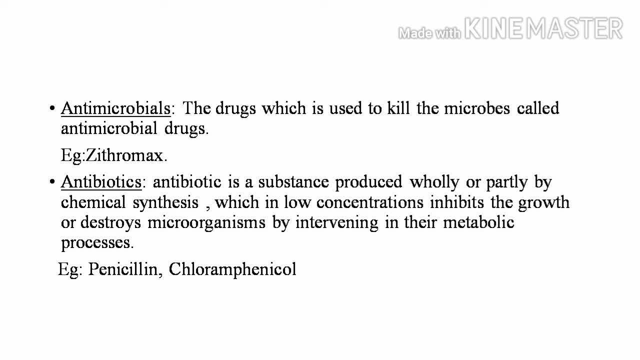 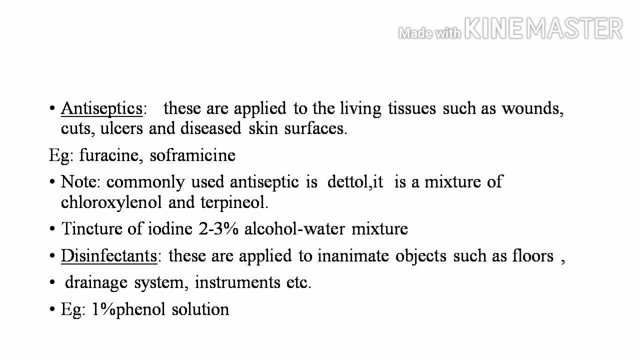 important antibiotic is chloramphicinol. Next, let us try to understand about antiseptic. I think so many of you have listened about this antiseptic. So what is antiseptic? These are applied to the body and the body is made up of a lot of things. So what is antiseptic? Antiseptic is a. 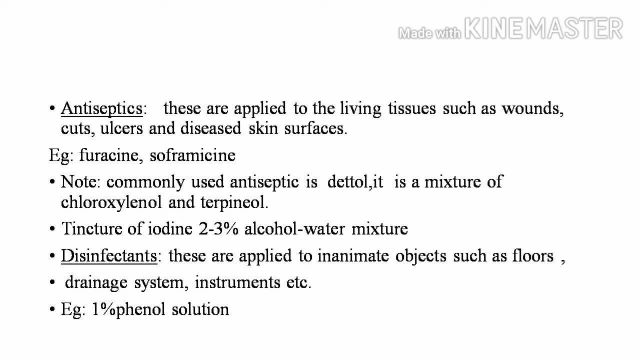 on the living tissues, such as wounds and cuts, ulcers and diseased skin surfaces. so what the role of this antiseptic? antiseptic are the drugs which prevent or which kill. the microbes which are occur on wounds or cuts are called as a antiseptic generally. when you have whenever our skin got cut. 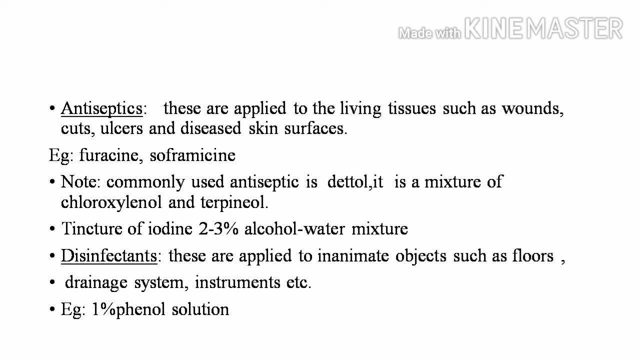 immediately our mother or in our school or PD sir immediately applies a Dettol on it. so what it will do? it does not allow the microbes get into our body. so the example of antiseptic is a furacin and soframicin. now, generally in our school or in our home we are going to use this Dettol. so what? 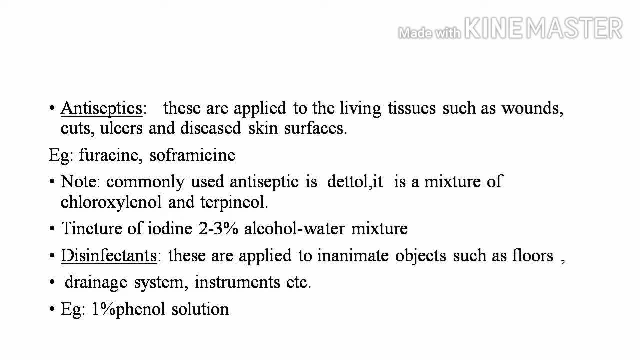 a Dettol consists of a Dettol is a mixture of a chloroxenol and terpenol, so chloroxenol and terpenol. sometimes we are going to use the tincture of iodine also, so this tincture of iodine is nothing but two to. 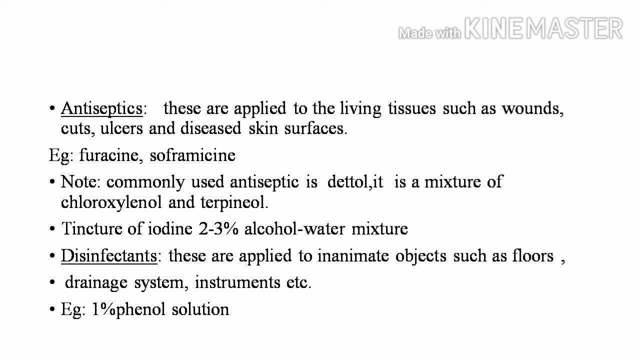 three percent alcohol water mixture. so tincture of iodine is two to three percent alcohol water mixture. next, let us try to understand about disinfectant. disinfectant: these are applied on intimate objects such as floor or drainage system or instrument. so many of you have gone. 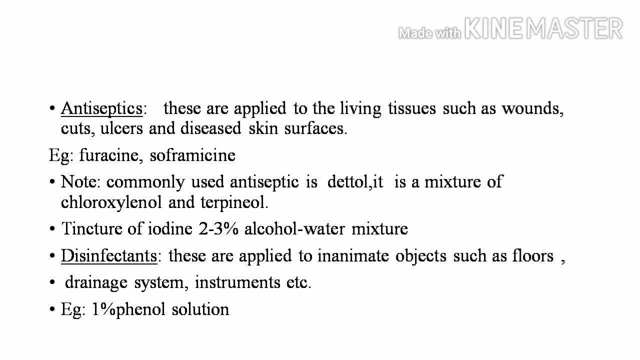 through this world, also disinfectant. so that difference between disinfectant and disinfectant is that disinfectant is applied on the living tissues, whereas disinfectants are applied on the non-living tissues. so disinfectants are applied on intimate objects such as floor or drainage system. 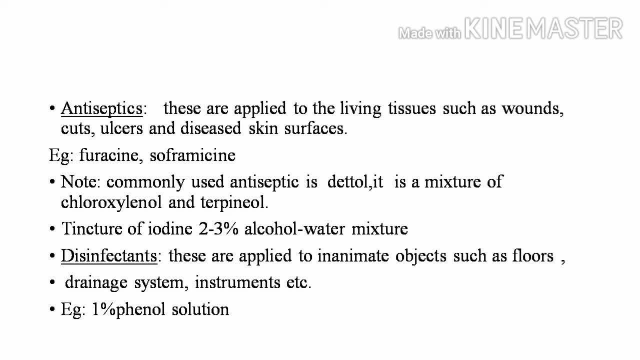 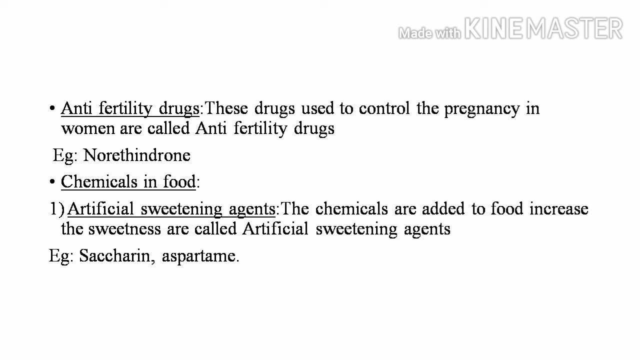 disinfectant also do the same work, which does not allow the growth of microorganisms. but disinfectants are applied on the floors- to today's system instrument and it does not- and all others- whereas antiseptics are applied on the living tissues. next let us try to understand. 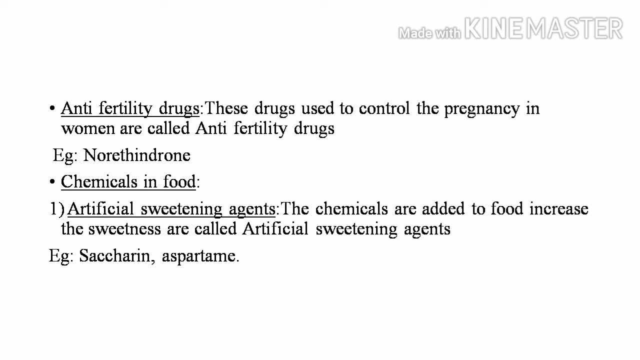 about anti-fertility drugs. i think all of you know about fertility. fertility means when sperm interact with ovum, it forms a zygote. the process is called as a fertility. in certain unexpected things may happen. so, in order to avoid the fertility, we are going to use 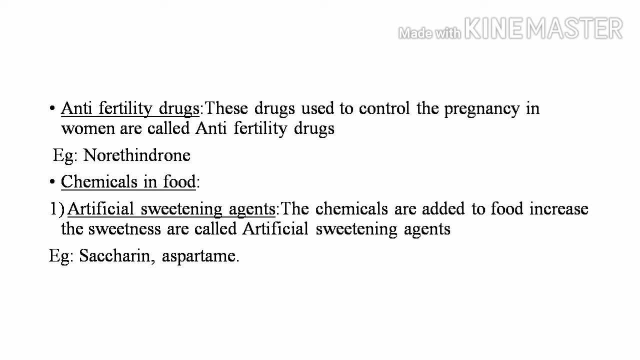 some drugs. those drugs are called as a anti-fertility drugs. so these drugs used to control the pregnancy in women are called anti-fertility drugs. i repeat: these drugs used to control the pregnancy in women are called anti-fertility drugs used to control the pregnancy in women are called anti-fertility drugs. 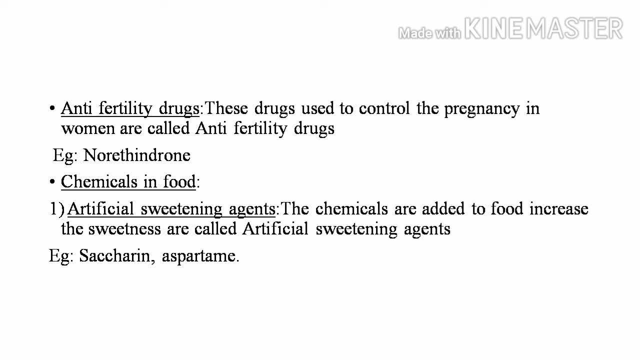 example of anti-fertility drugs is nown ethinker on. next let us try to understand about another important classification of chemistry in everyday life, that is, a chemicals in food. in that first let us try to understand about artificial myself, because in the, indeed in animal's blood, the chiral circulation is important. 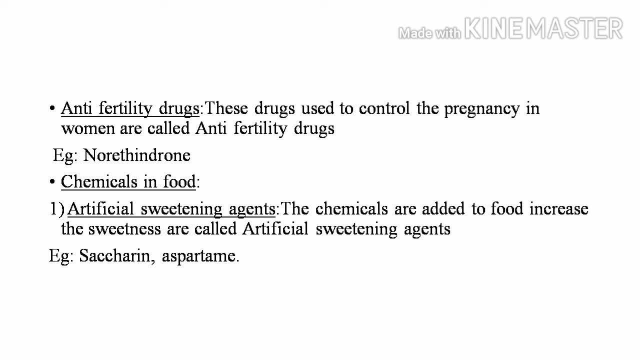 agents. the chemicals are added to food to increase date of life. so every gram mixture and so that is called ant emergedGAN 나온출지, So the toxic chemical of ذ MIN reduction done in to our fluid for an artificial. These sweetness are called artificial sweetening agents. 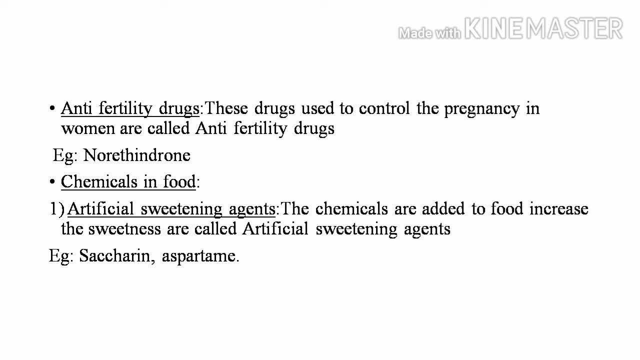 I think so many of you have seen. sugar patients are using certain tablets in order to have the sweetness. So what they are going to do, they gives the sweet taste but they do not increase the glucose level in the blood. So those are called as artificial sweetening agents. 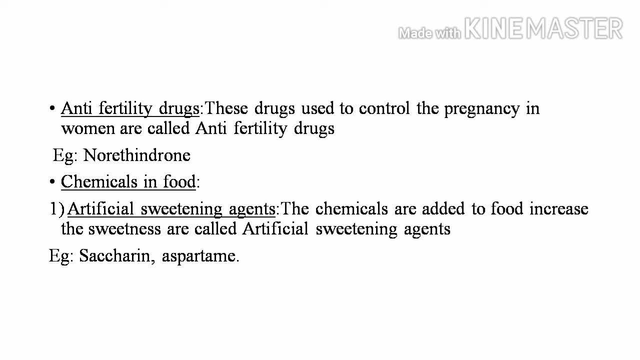 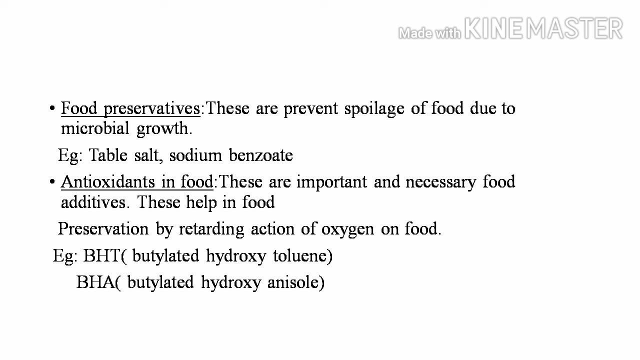 So I repeat, the chemicals are added to food to increase the sweetness are called artificial sweetening agents. Example of artificial sweetening agents are sacherin and aspartame. Next, let us try to understand about food preservatives. When the food is kept outside for long time we are going to have a very bad odor. that 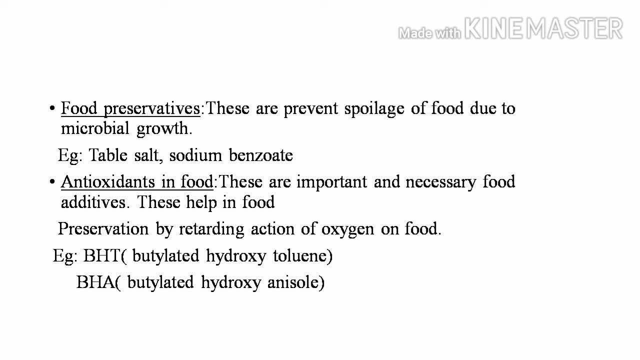 indicates the food get poisoned Or the food is spoiled. In order to avoid that, we are going to add certain chemicals. Those chemicals are called as a food preservatives. These are prevent spoilage of food due to microbial growth. Generally, in order to store the pickles for long time, sufficient quantity of salt is added. 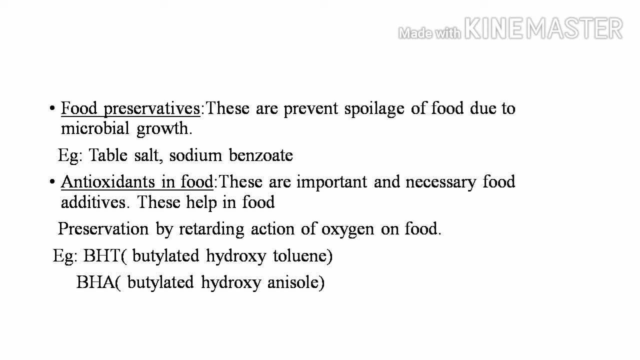 That salt does not allow the growth of microbial growth. uh, it preserve the pickle for long time. the example of food preservatives is a table salt. next, let us try to understand about antioxidants in food. when the apple is cut, when it is kept it outside after some time, the color of apple changes in the same way. 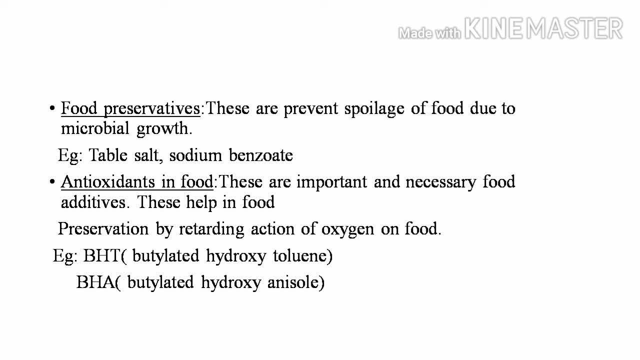 whenever a fruit is cut into half and kept it outside after some time, the color get tarnished because of oxidation. so in order to avoid that, certain chemicals are added- those are called as antioxidants in food. these are important and necessary food additives which prevent oxidation of food. example of 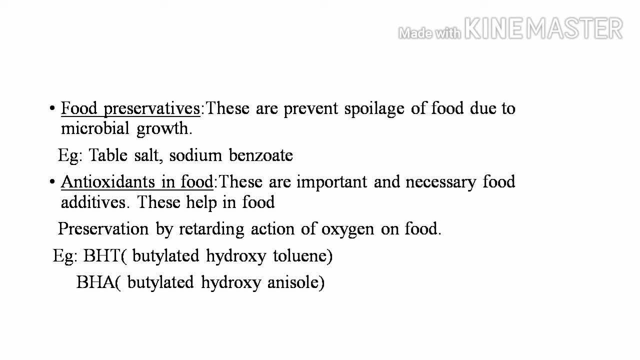 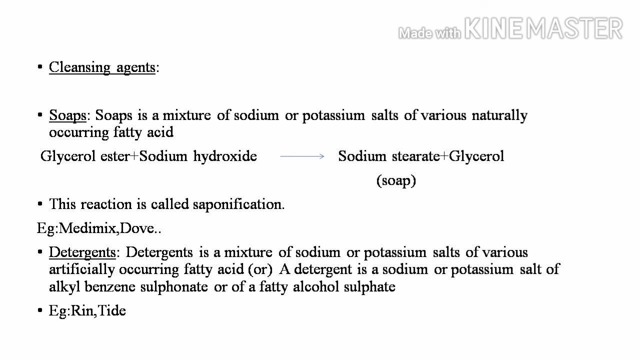 antioxidants in food are BHT and a BHA. the full form of BHT is a butylated hydroxy toluene and a butylated hydroxy anyzole. next, let us try to understand about another important category in chemistry in everyday life. those are cleaning agent generally in order to clean our body. as well as in order to clean the dirty clothes. we have to use a lot of water and oil to clean our body, because our body is made of water, so we will have to use a lot of water and oil, as well as we have to use a lot of water to clean our body. 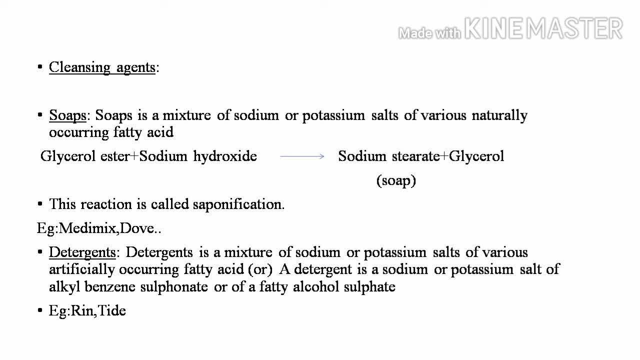 are going to use a surf medimix and all others. first let us try to understand about soaps. soap is a mixture of sodium or potassium salt of various naturally occurring fatty acids. understand this word naturally occurring fatty acids? so soaps are made by adding a sodium. 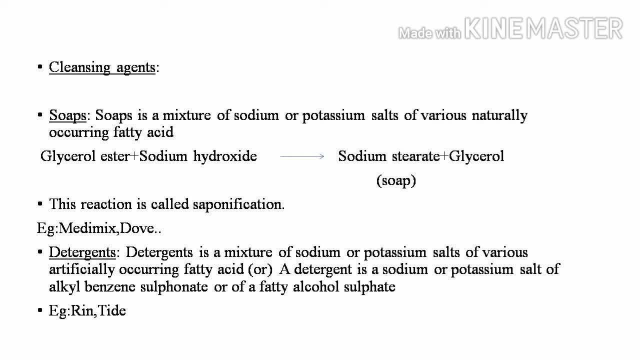 hydroxide to triglycerol, which results in the formation of sodium stearate and glycerol. that sodium stearate is called as a soap and this reaction is called as a saponification. this phenomena you have learned already in 10th class. the example of soaps are medimix and 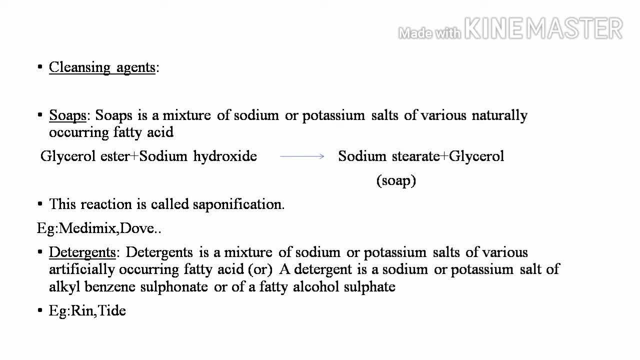 dow. next, let us try to understand about detergent. detergent is a mixture of sodium or potassium salt of various soaps artificially occurring fatty acid. in case of soap, soap is a mixture of sodium or potassium salt of various naturally occurring fatty acids, whereas in case of detergent, detergent is a. 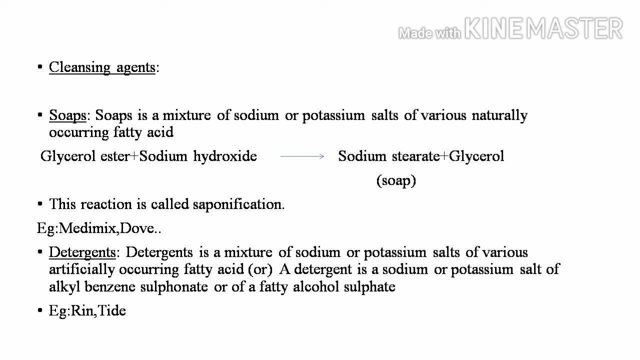 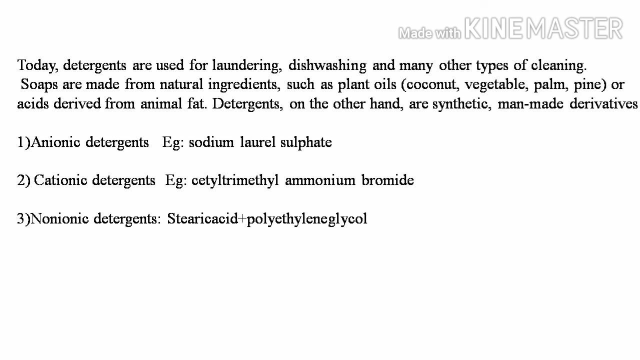 mixture of sodium or potassium salt of various artificially occurring fatty acid. so detergents are made from artificially occurring fatty acids, whereas soaps are made from naturally occurring fatty acids. example of detergent is a. nonела is a mixture of naturalредs backbone fat, glyphosate, neutron monosaccharide or